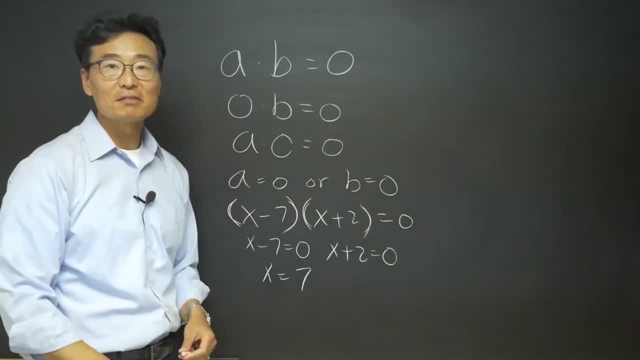 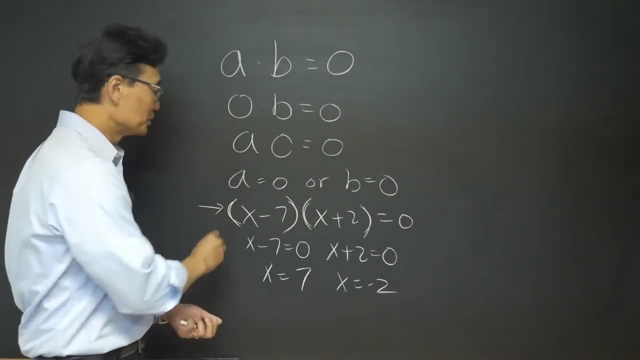 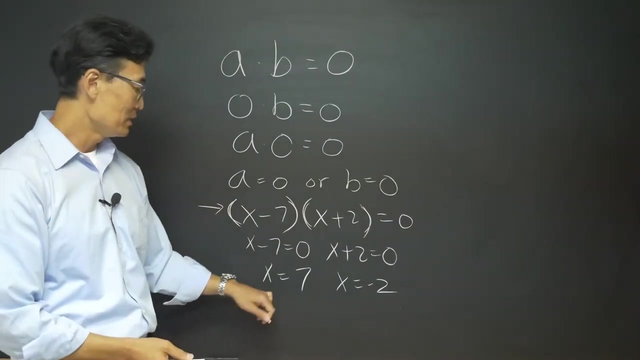 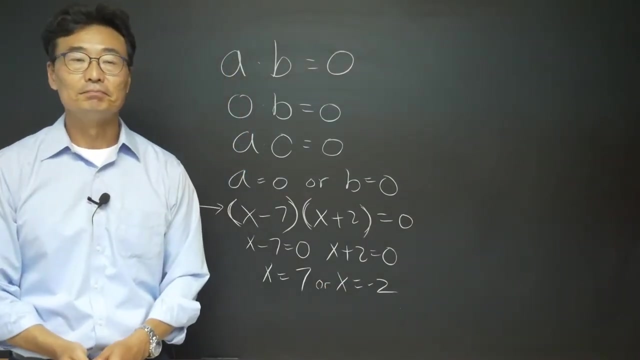 solve: we get X equals to seven from this and we get X equals to negative two from that. So if we were given this equation, parentheses X minus seven times parentheses X plus two equals zero. then X is either seven or negative two. So let me go ahead and do a couple more examples. 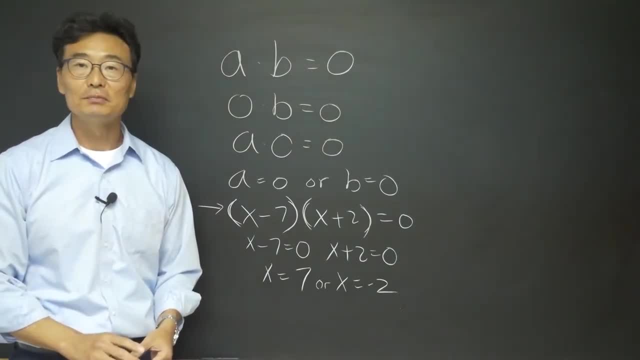 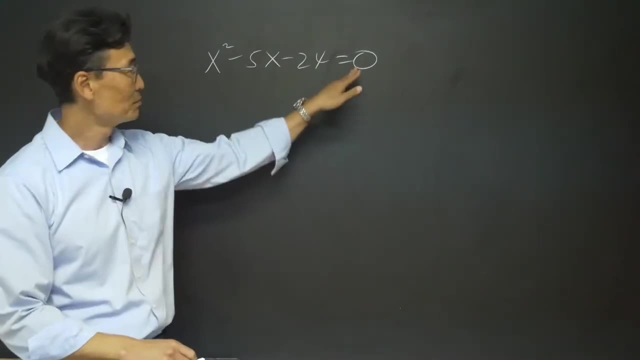 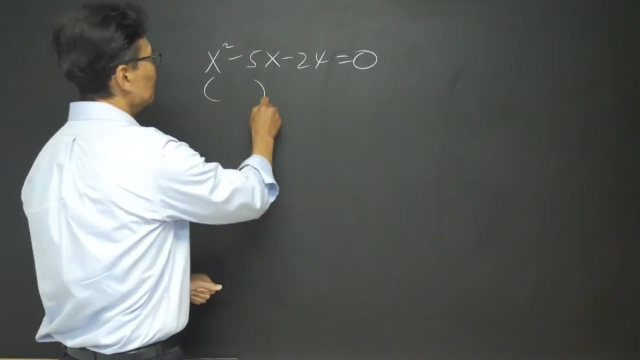 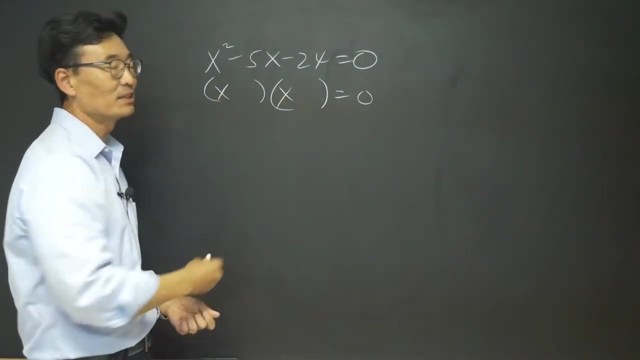 a quadratic function To show you how we could use this. Here's a pretty standard quadratic equation, set equal to zero, To solve for X. what we're going to do is first factor this: If we factor X squared minus five, X minus 24, we're going to start with X and X and then, since the sine is negative, the third one. 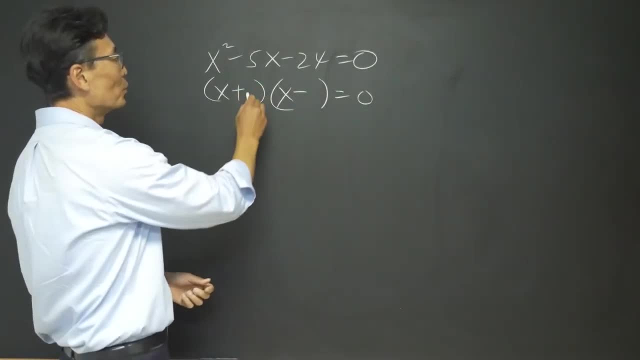 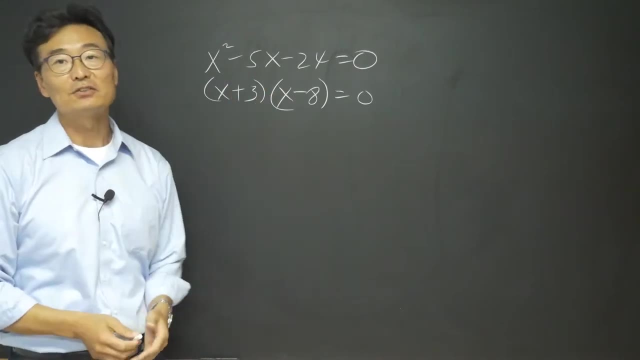 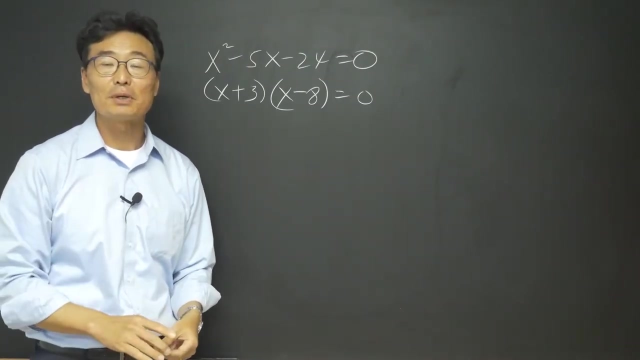 we're going to start with X To get a difference of five. we're going to go with three here and eight here. Learning to factor is part of algebra one, which is not covered in my lessons, but it's something you might want to go back to algebra one and practice, because you do need to be able. 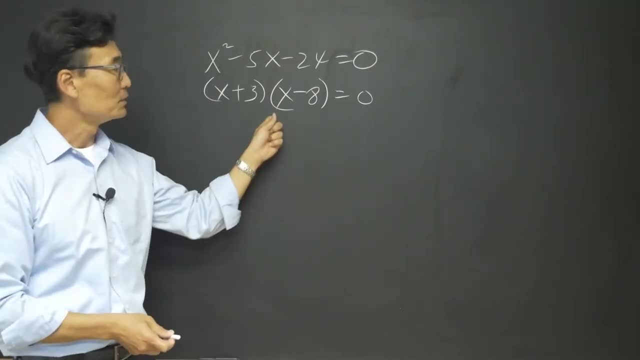 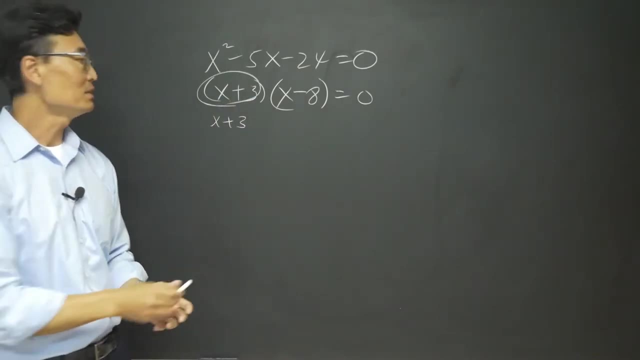 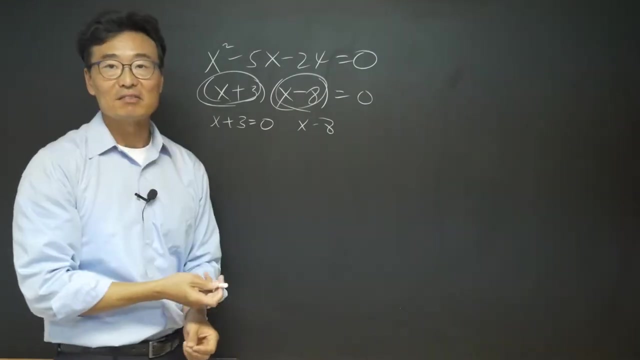 to factor a quadratic equation into this format, Then from this we know that either X plus three, meaning the first parenthesis, is going to be negative, So we're going to start with X plus three, which is going to equal to zero, or X minus eight, meaning the second parenthesis portion is equal to. 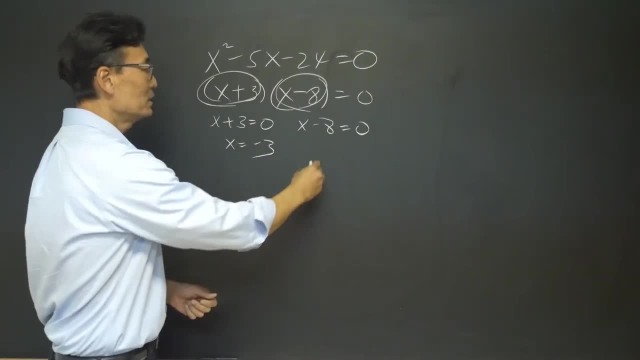 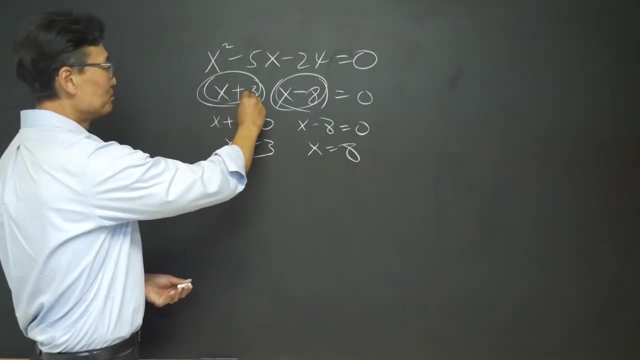 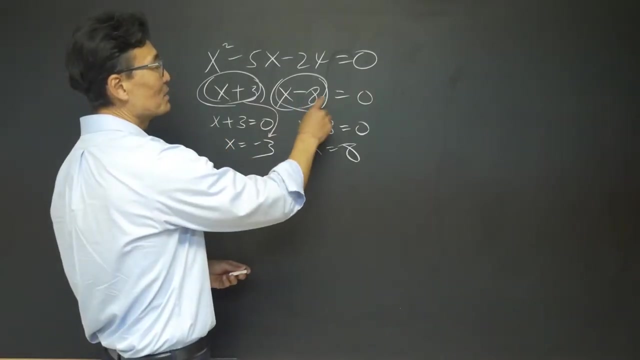 zero. So we get either X equals negative three or X equals to positive eight. And of course you notice that when we have that positive three it's negative three here, for obvious reasons, because we solve for that. And then if it's X minus eight, X equals two positive eight, It's the opposite. 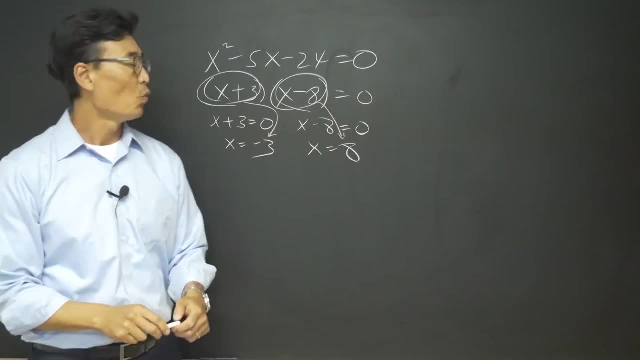 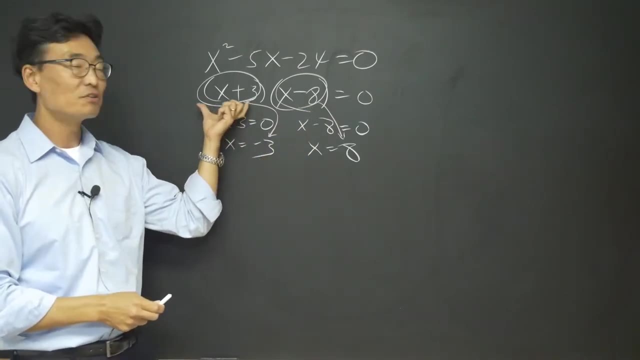 of zero, So that's going to be negative three, So that's going to be positive eight. And then if it's sign. But it's better to understand why the signs are different rather than just memorizing the changing the signs. It's because we take whatever is in the 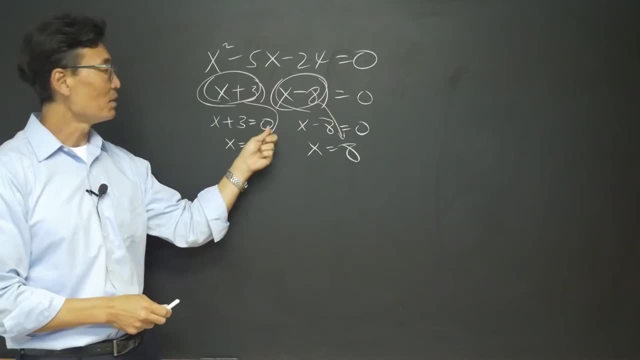 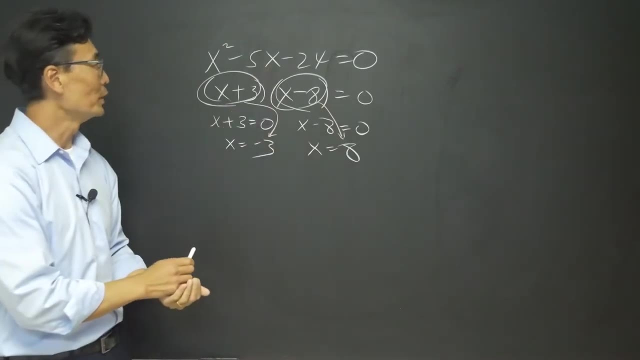 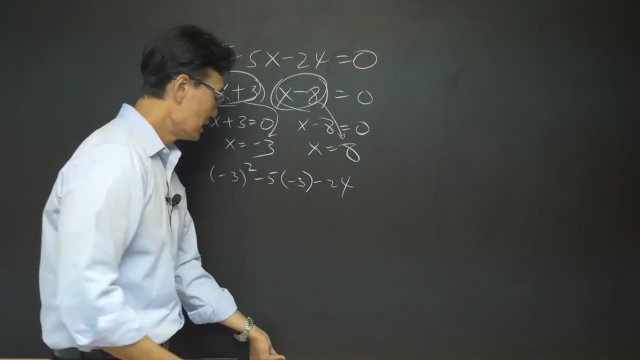 parentheses, set it equal to 0, and then, solving it, give us the answer. So if we were to take negative 3 into this equation, negative 3 squared minus 5 times negative 3 minus 24, and I did plug this in the calculator and you do. 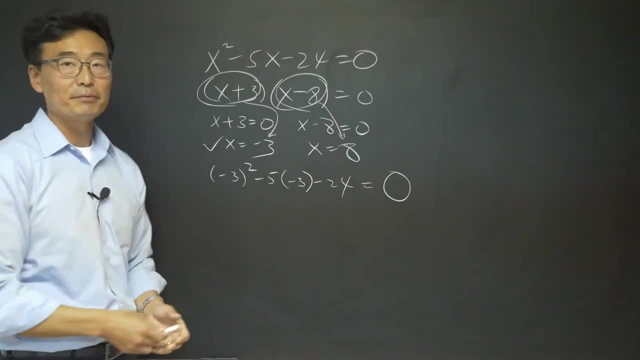 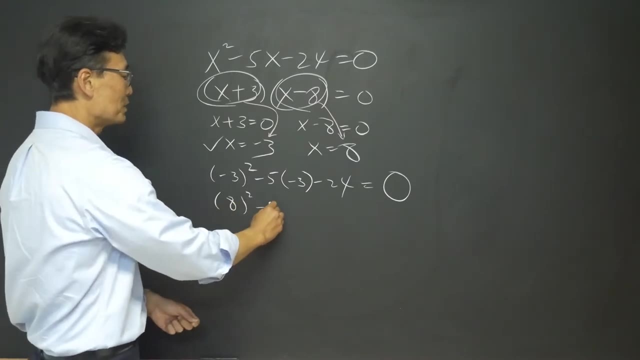 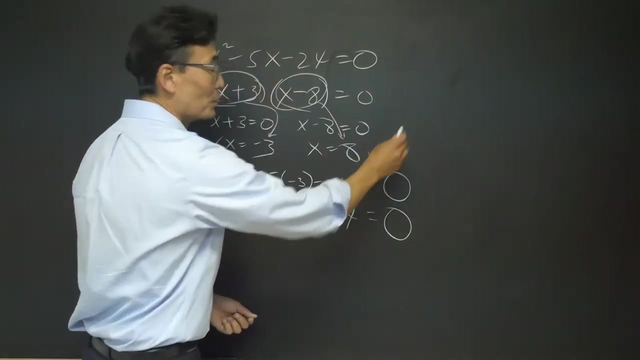 get 0.. So we know that negative 3 works for sure, and this is how you go about checking your answers. And then, if we take the 8, meaning 8 squared minus 5 times 8 minus 24,, once again you get 0 as well. So we know that 8 is an answer as. 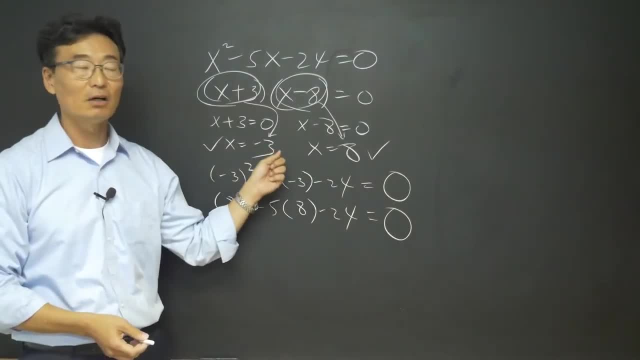 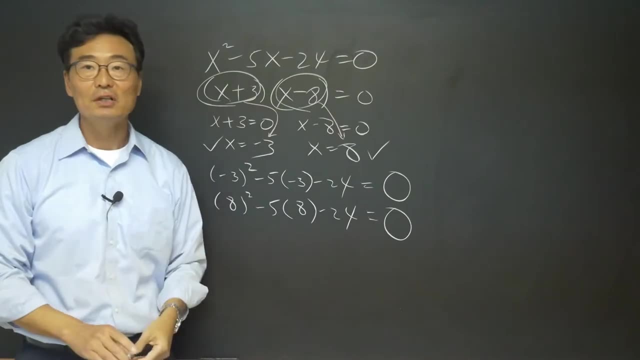 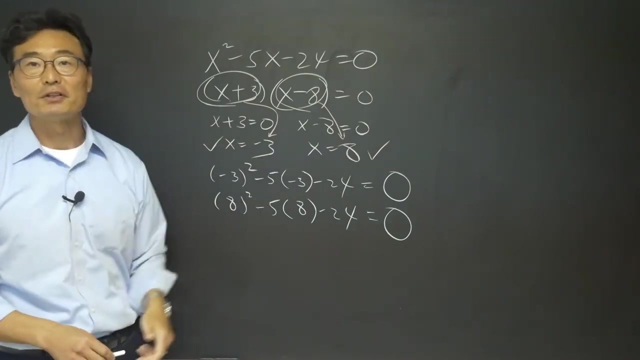 well, So if you want to check the answers that you've gotten, I'll always go ahead and plug it into the original equation, like I just did, and then see that they are equal to 0, thereby confirming the fact that these two numbers are the answers. Okay, Alright, let me do another one over here on the side. 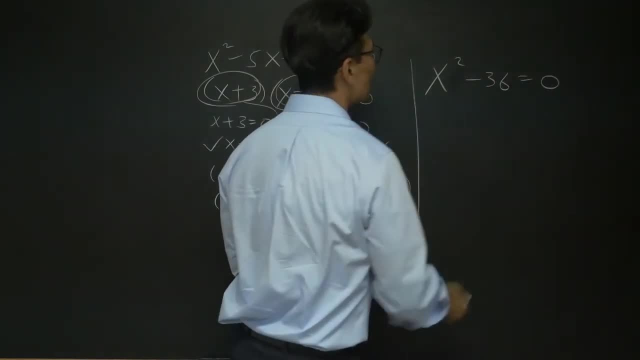 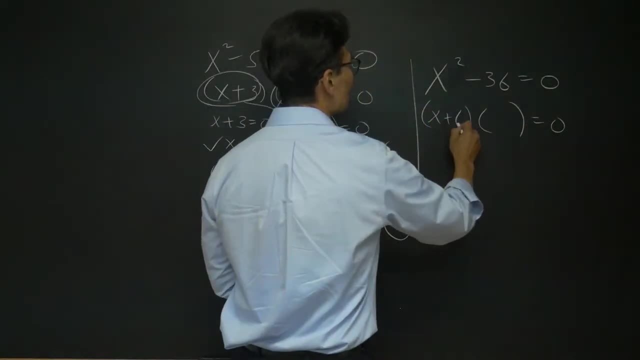 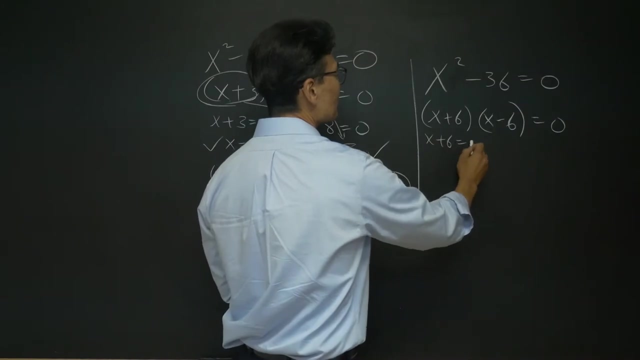 What if the question said: to solve for x squared minus 36?? Let's go ahead and factor this once again. It's going to be x plus 6,, x minus 6.. Again, take what's in the first parentheses, set it equal to 0, and also. 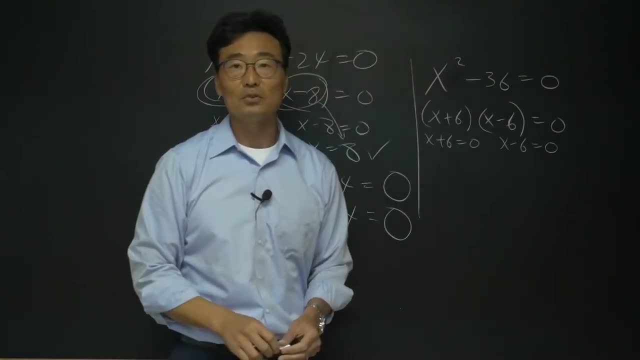 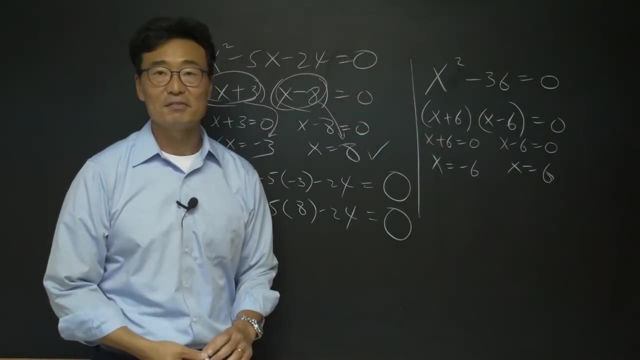 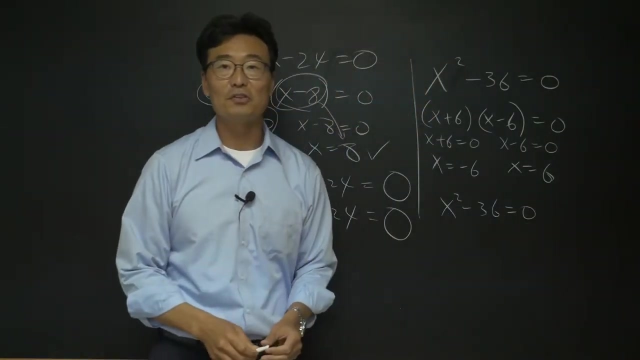 take what's in the second parentheses and set it equal to 0 and solve. Then we get x equals to negative 6 and x equals to positive 6.. If you remember, when you have x squared, minus 36 is equal to 0, another way, the way we've done it in our 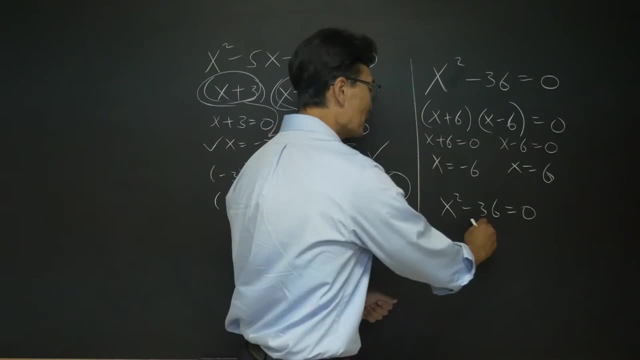 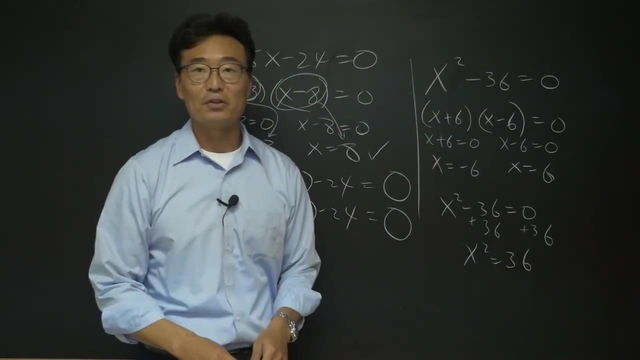 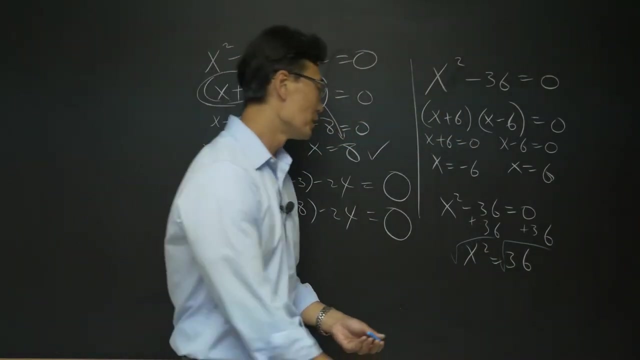 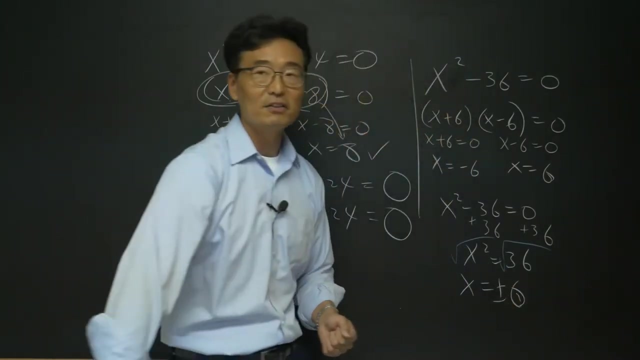 other sections and in previous sections is that you go ahead and add 36 to the left and the right side, giving us x squared equals to 36, and then taking the square root of the left and the right side, Then we end up getting x is equal to square root of 36 is 6, but don't forget the plus minus. 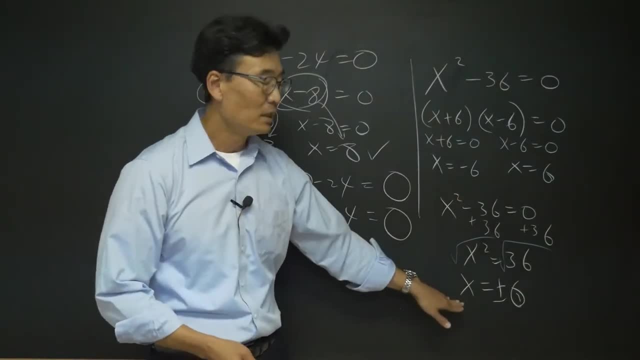 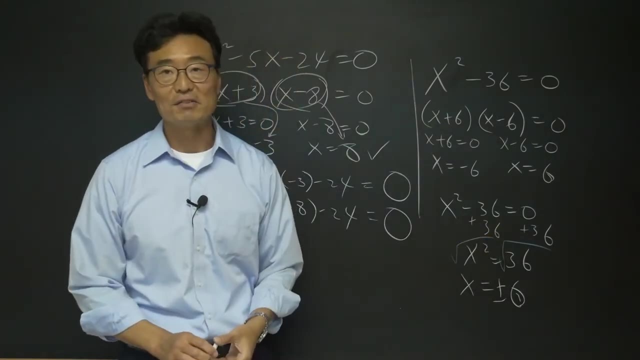 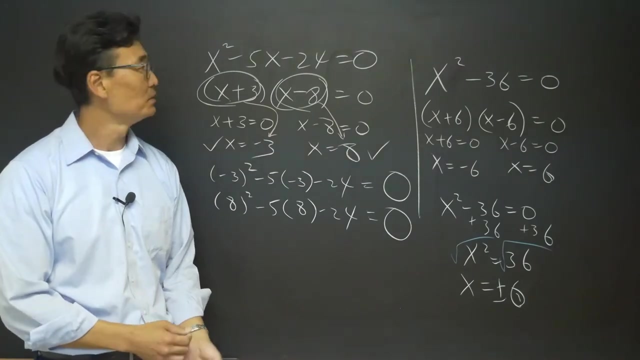 wherever you take the square root, giving us the same answer. Okay, So that shows that this method works as well. So that's a another way of checking your answers. Alright, so let me do a couple more different ones that are a little bit more difficult. solving quadratic equations using factoring. 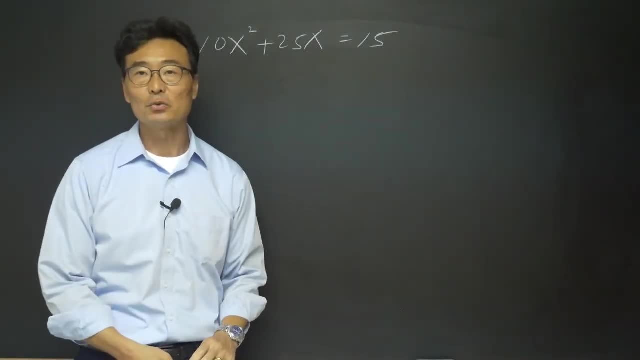 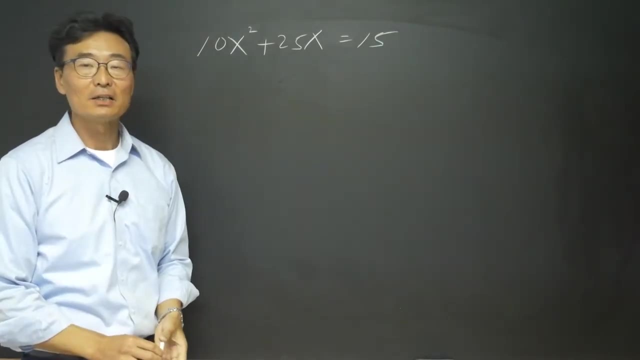 method. Here's a more challenging question. Notice again: we have a quadratic equation. However, the right side of the equal sign is not equal to 0 and it's equal to 15.. So the first step always is to make the right side or the left side, one or the other. 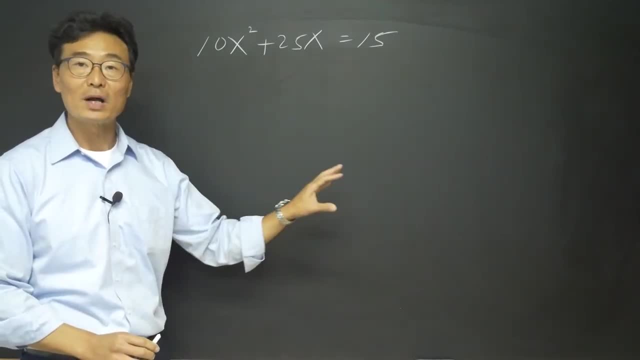 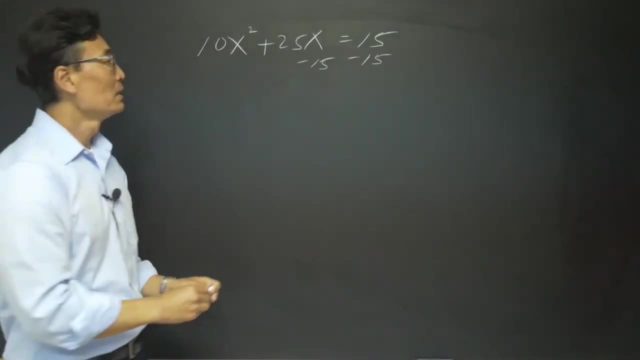 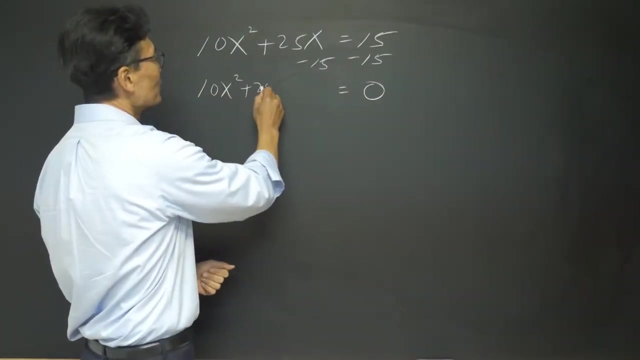 equal to 0.. In this case it's pretty obvious that we want to make the right side equal to 0 by subtracting 15 from the left and the right. Then, of course, we get a 0 on the right side of the equal sign and we get 10x squared plus 25x, minus 15 on the left side. 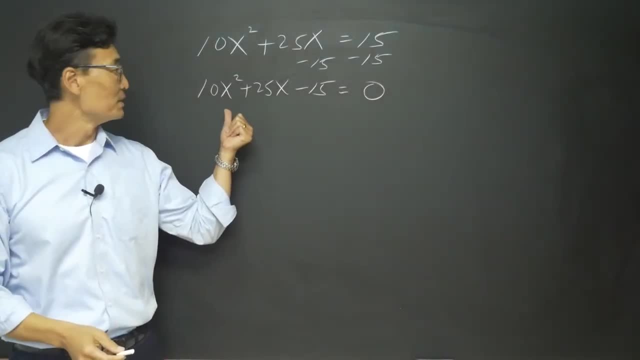 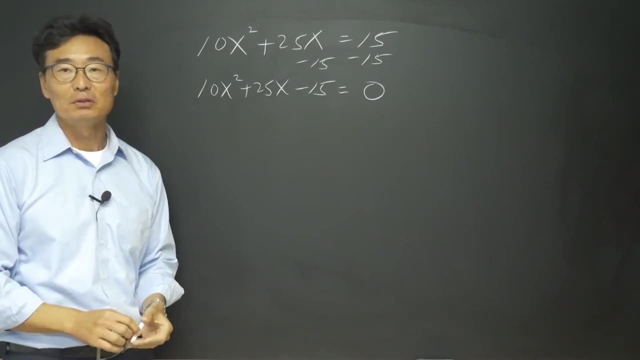 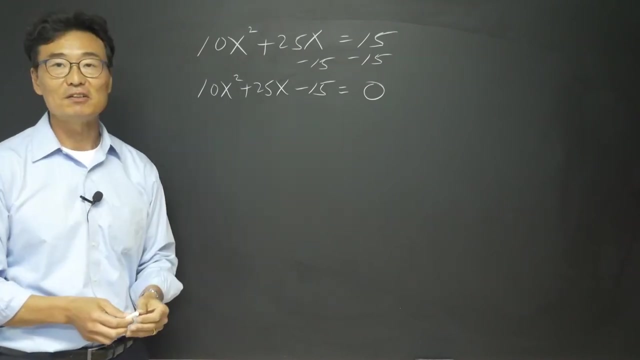 of the equal sign, Although we could factor this equation right away, straight up. but when the numbers are big, it makes the factoring process more difficult. So what you want to do is, whenever you could factor out a number, a number from three places here, then you want to do that And I'll show. 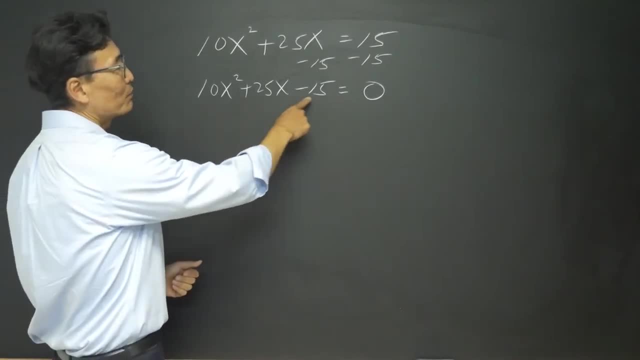 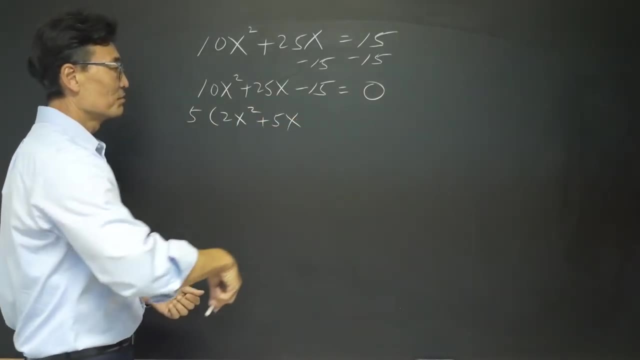 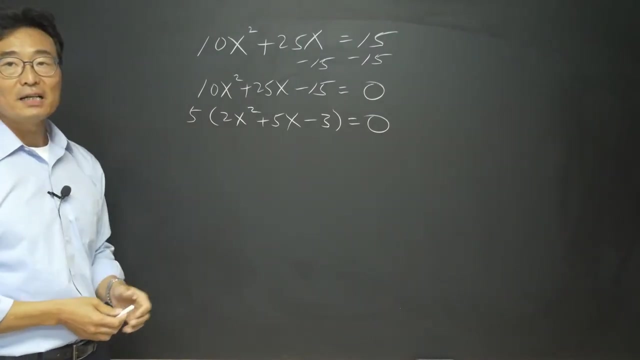 you why? What can we factor out from 10,, 25, and negative 15?? We could take out a 5, giving us 2x squared plus 5x minus 3.. And what do we do with that 5?? We could actually go ahead. 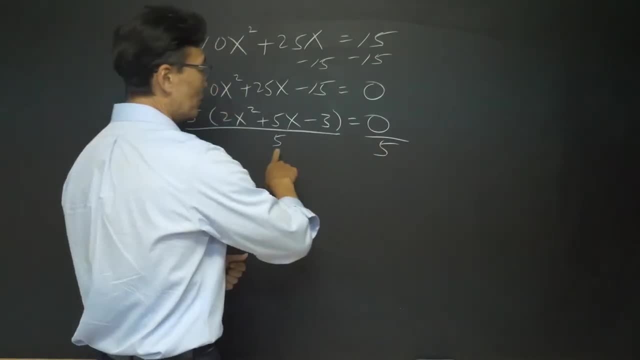 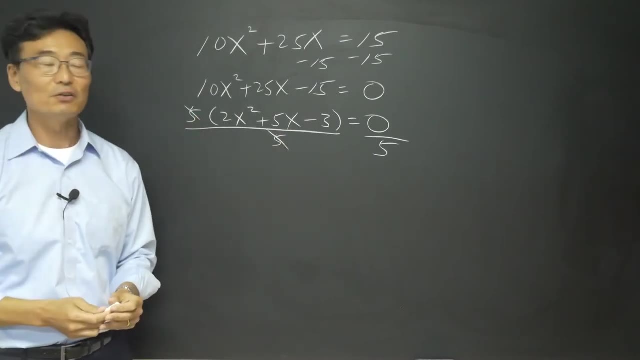 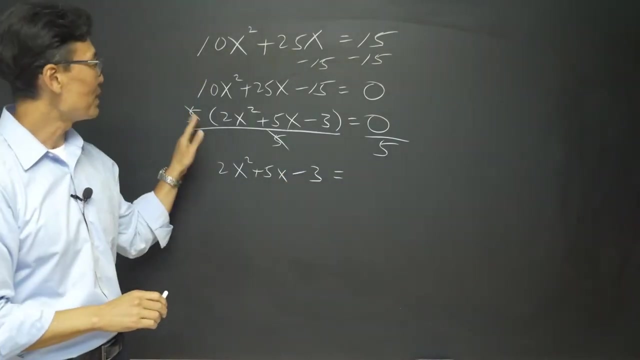 and divide it by 5 on the right or the left and the right, both the left and the right side. By doing so, the 5 in the front cancels out, leaving us with only 2x squared plus 5x minus 3.. And the beauty of this: factoring out the 5 and dividing it by 5 on the left. 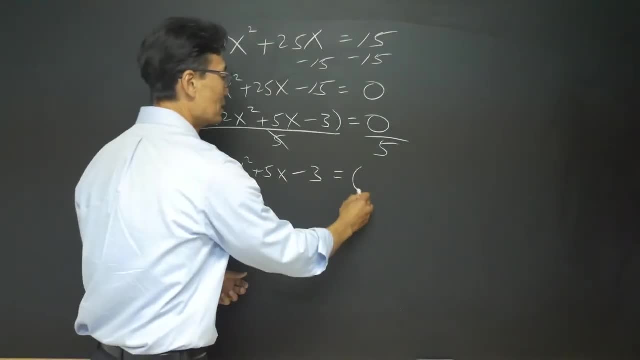 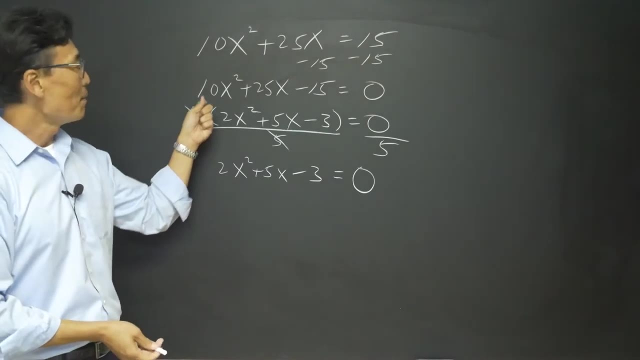 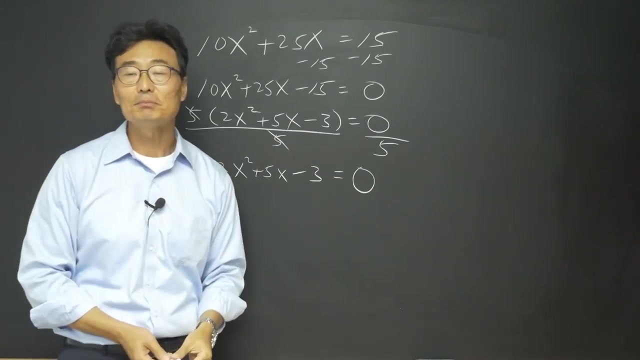 side and the right side is that 0 over 5 is of course, 0. That way we get to keep the 0. on the right side, We get rid of the 5.. make the numbers smaller. From 10,, 25, and 15, we made it into 2,, 5, and 3.. It's a pretty nice way to simplify your work. 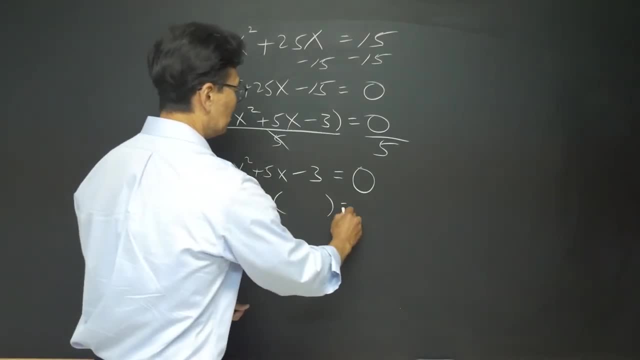 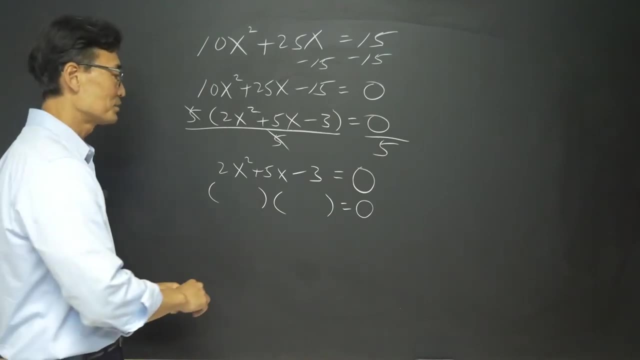 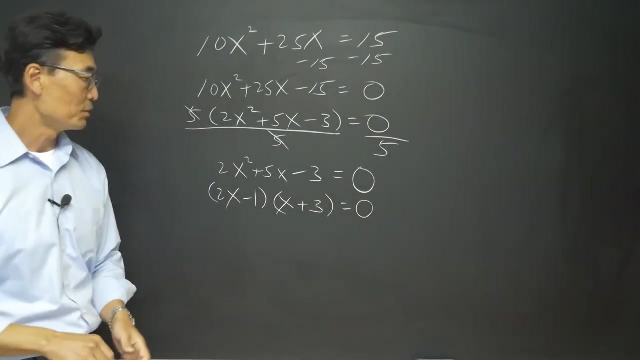 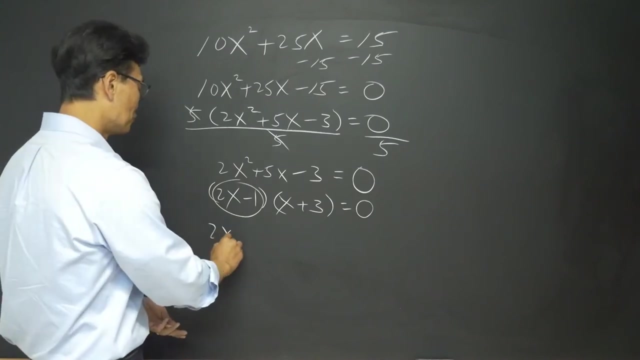 Now let's go ahead and factor this Again. factoring wise. there are many methods, but I'll just skip the process and just go ahead and factor it right away. So we get 2x and x plus 3 here and minus 1 here. Once again, we're going to take whatever is in the first parenthesis, 2x minus 1, set it equal to 0.